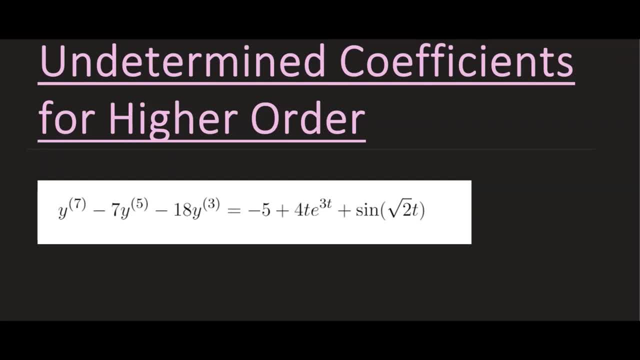 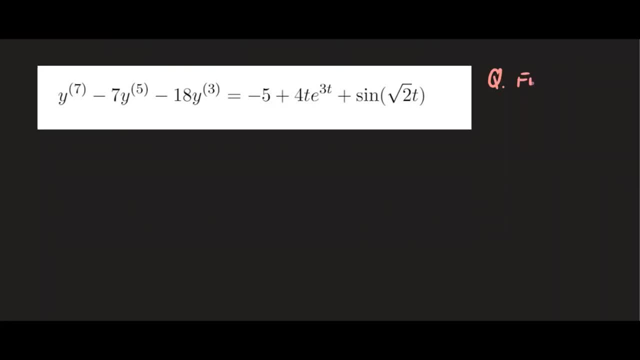 the homogeneous case. So let's go ahead and do that. So we're going to. so the question for this problem is to find the form of the particular solution. So we want to go ahead and find the homogeneous solution first. So let's do that. 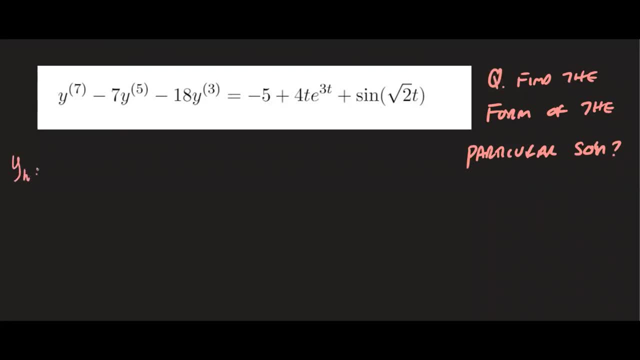 So we are looking for y sub h, So we're going to set the equation equal to zero. So we have y to the seventh derivative minus seven, y to the fifth derivative minus 18, y to the third derivative equals to zero. So now we go ahead and write out the characteristic. 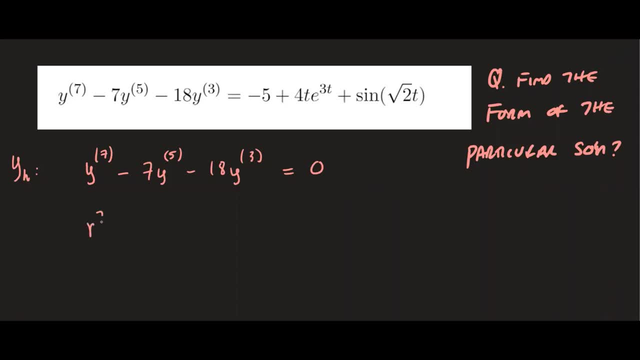 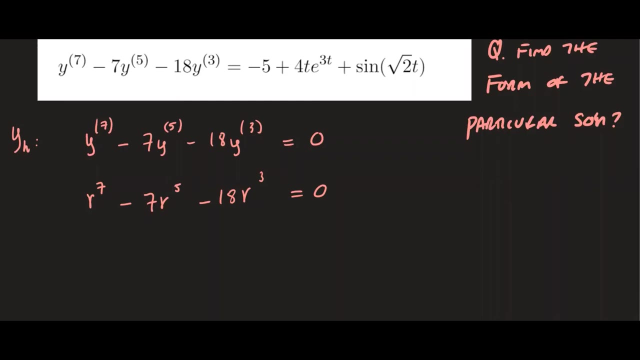 polynomial. So we have r to the seventh power minus seven, r to the fifth minus 18.. r to the third equals to zero. And then we use factoring to find the roots of this polynomial. So we have cube times: r to the fourth minus seven, r squared minus 18 equals to zero. And 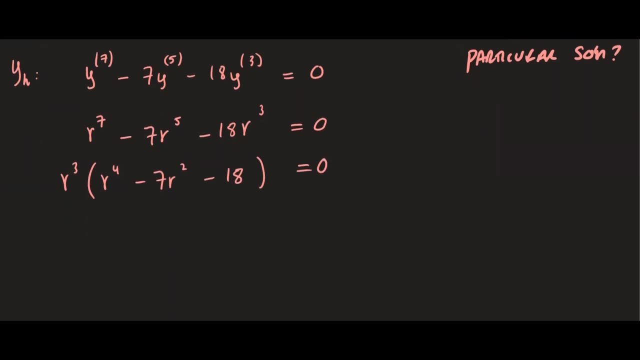 then the parenthesis portion can be factored a little bit more, So we still have our cube outside, And then we can factor the inside with: r to the fourth minus seven, r to the fifth plus seven, r squared minus nine, And then r squared plus two. So that way this can be. 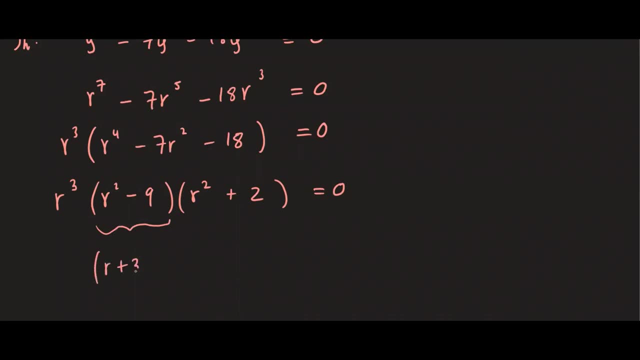 factored a little bit more, That would be r plus three and then r minus three, And we still have our cube And we have r squared plus two equals to zero. So that will give us all the roots. So from this one, if we set it to zero, our cube equal to zero. 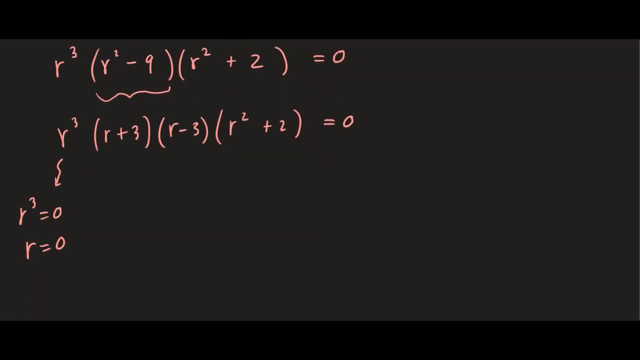 that gives us r equal to zero. So we have three repeated roots from this one. So we can say: r one, r two and r three are going to be zero. So those are the repeated roots with zero. And then we can say, for instance: if we set this one to zero, we get r four. let's call it. 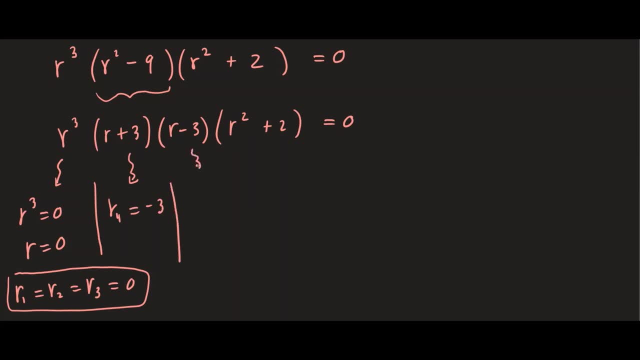 equals to negative three. And then if we set this one to zero, we have r five equals to three. And then if we set this one to 0, we get, say r squared is equal to negative 2.. And then take the square roots, you get complex roots. 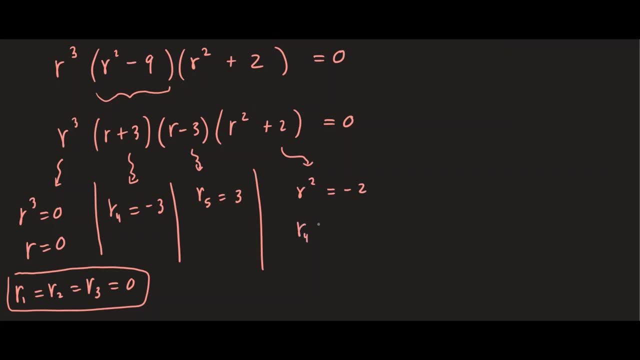 So we have r4, sorry, not r4, r6 and r7, which are complex conjugate of plus and minus, square root of 2i. So 6 and r6 and r7 are complex conjugate. So now we're ready to write down the homogeneous solution to this equation. 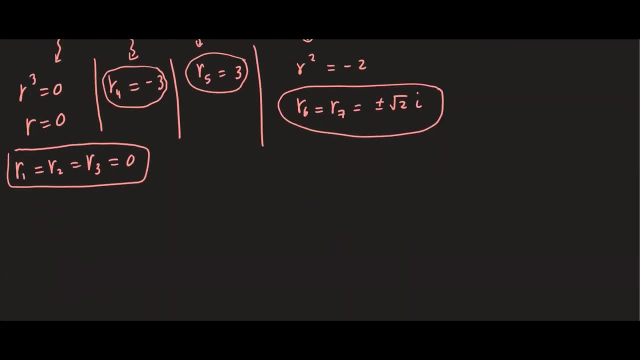 So these are the roots. So we have, from the first, r1,, r2,, r3,. our solution is going to be c1, e to the 0, which is 1, plus c2.. Now to make them two distinct, we multiply it by t. 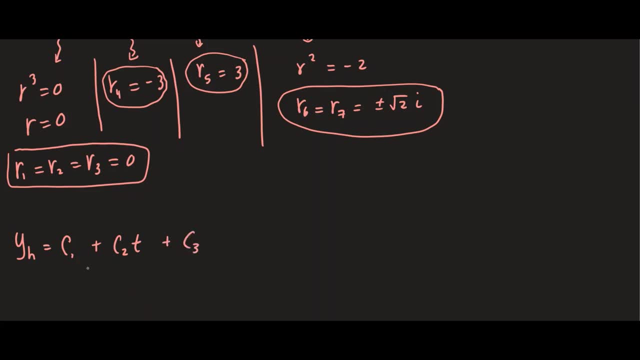 Plus c3, now make this one distinct from the previous two. We multiply. We multiply with t squared, So these are the three coming from: r1, r2, and r3.. Now, with r4, we have real roots. So that's going to be c4. e to the negative 3t. 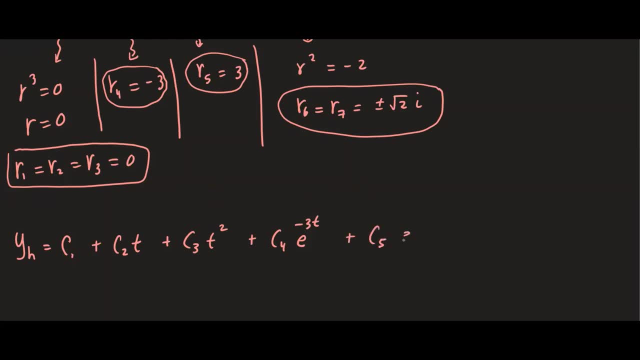 And then c5 coming from r5, that's e to the 3t, And then the last two are going to be complex conjugate where beta is square root of 2.. So we have plus c6.. Cosine of a square root of 2t, plus c7, sine of a square root of 2t. 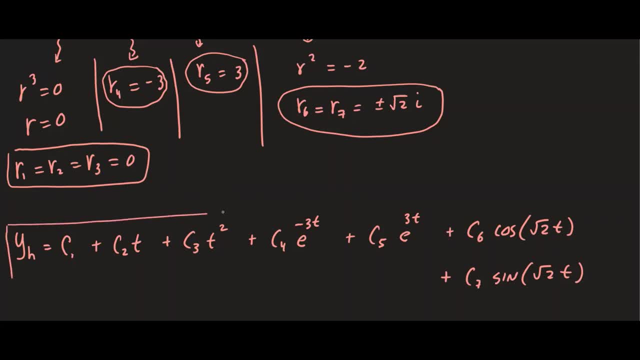 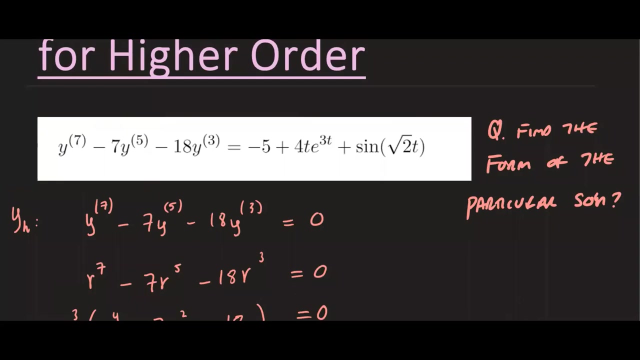 So there we have our homogeneous solution. Well, now we have to figure out what could be the possible form of the particular solution based on the non-homogeneous equation. So we look at the right-hand side of this equation. So we We need a form for this piece. 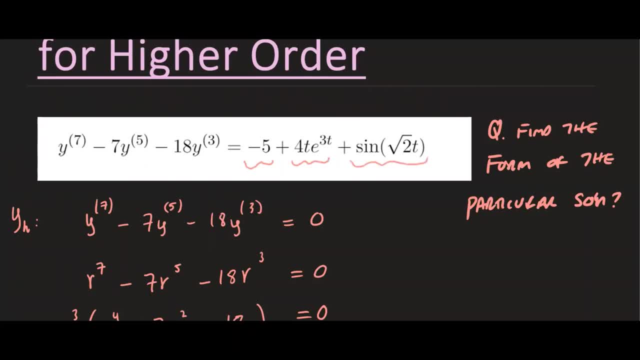 We need a form for this one And we need a form for that one. So let's go ahead and label these. What are those different forms we're going to be using? So let's call this: particular solution form 1, particular solution form 2, particular solution: form 3.. 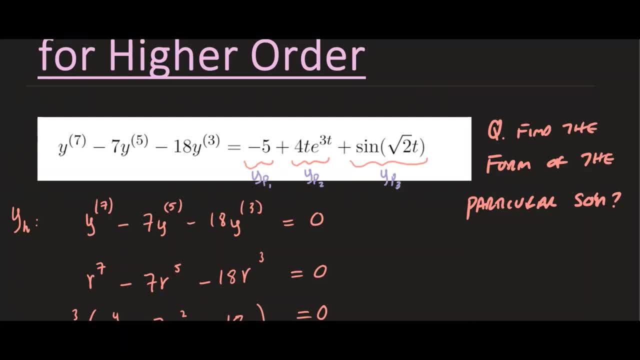 And then we'll try to use our homogeneous case in there. So yp1 is a constant term negative 5. So it's a polynomial. So it's a polynomial of degree 0. So let's call it a constant. So yp1 has to be just a constant. 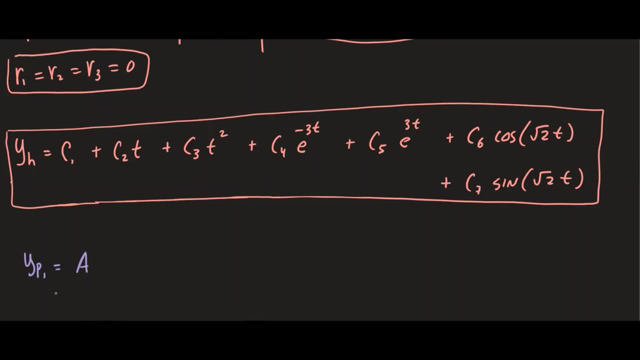 So that's a. Now we want to make this one independent of the homogeneous case, So it looks like it's going to duplicate with this one. If I multiply it by t, then there is a duplication here. If I multiply it by t squared, there is a duplication here. 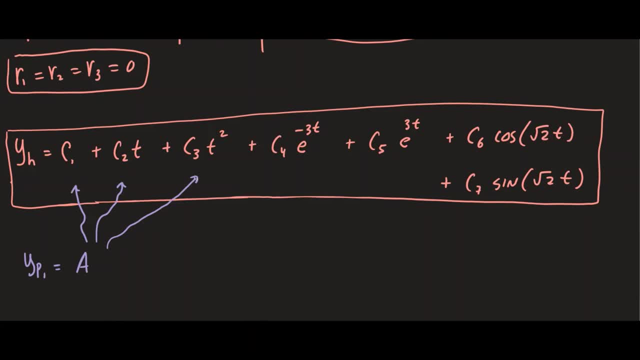 So that we don't overlap with the homogeneous, I must Multiply this function with tq. That way there are no duplication in the homogeneous with the particular solution form. So that will be the form for the first particular function. Now what about for yp2?? 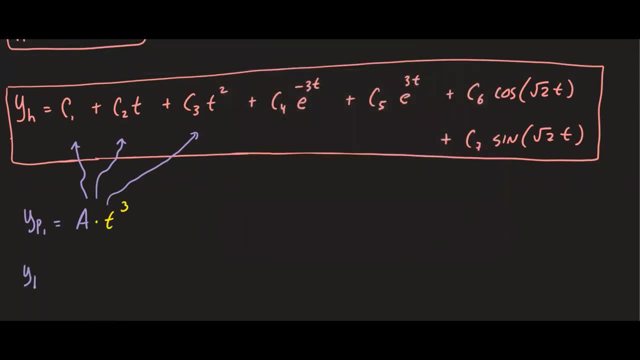 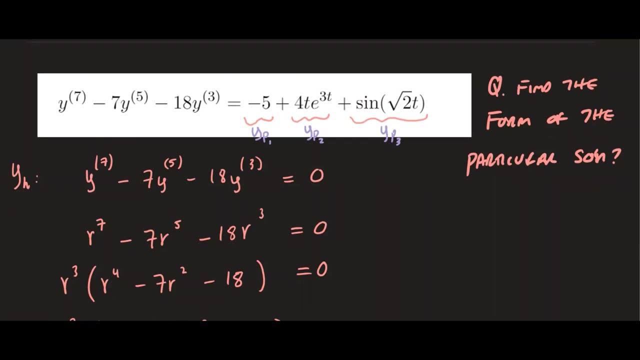 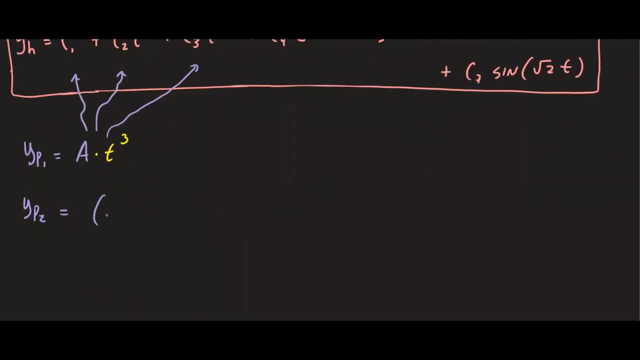 So let's take a look at what yp2 was. So yp2 is a linear times the exponential 3t. So we need a linear and the exponential 3t So we need a linear. So that would be, let's call it, bt plus c and the exponential e to the 3t. 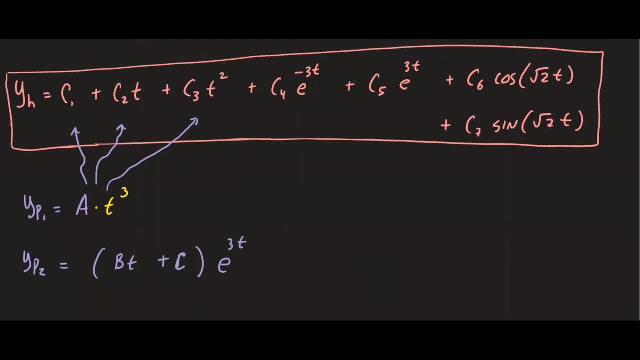 Well, now let's check: does this have a duplicate in the homogeneous? If I distribute this, my function- that I'm guessing- is pretty much bt, e to the 3t plus c e to the 3t. That's what I'm guessing. 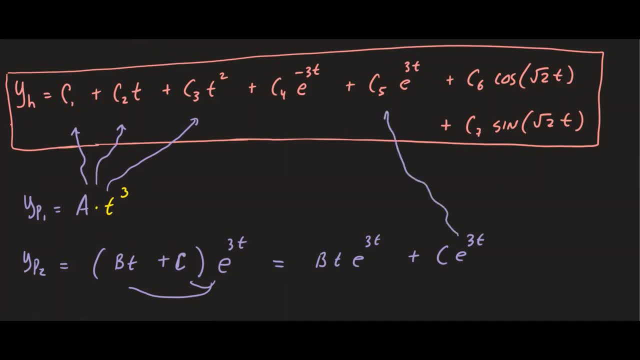 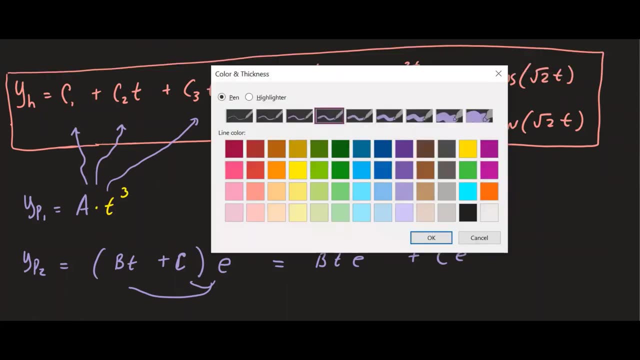 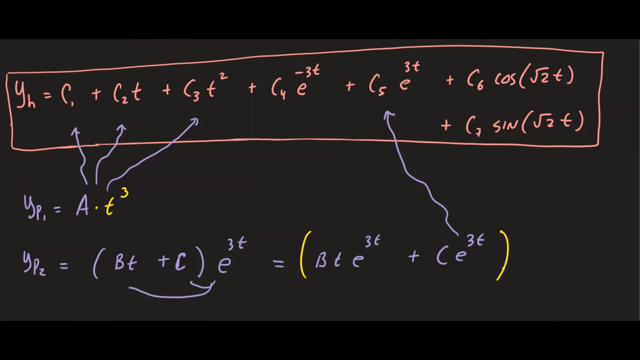 Now it looks like this one has a duplication right here. It's exactly the same, except for the constant, which is not a big deal. So that means I must modify this guess by multiplying it by some t to some power. So it looks like if I multiply this by t, that will remove the duplication. 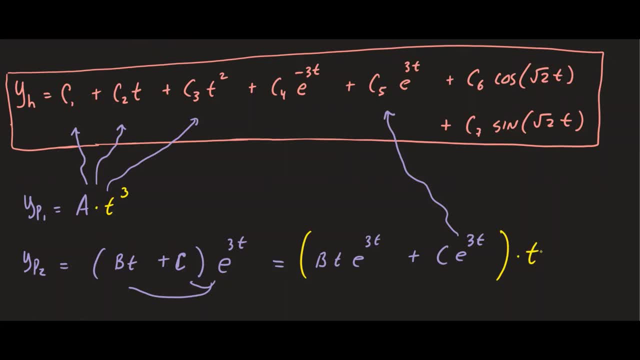 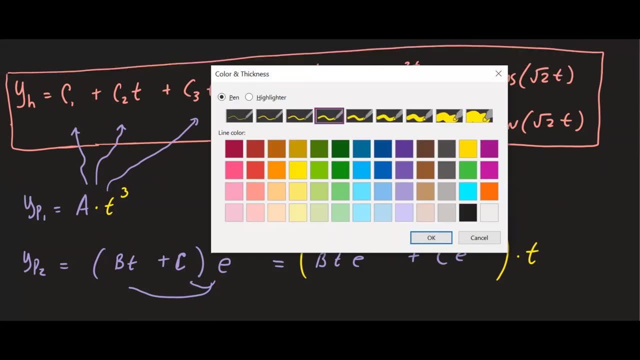 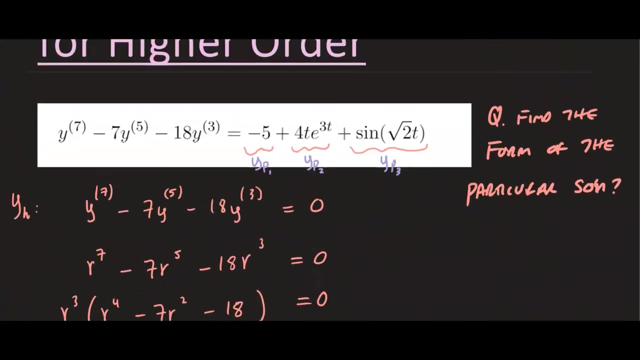 So we're good to go with yp2.. So my yp2 would be this: function times t, And then that will remove the duplication. And the last function we're looking at is yp3.. So let's check what yp3 we're guessing.